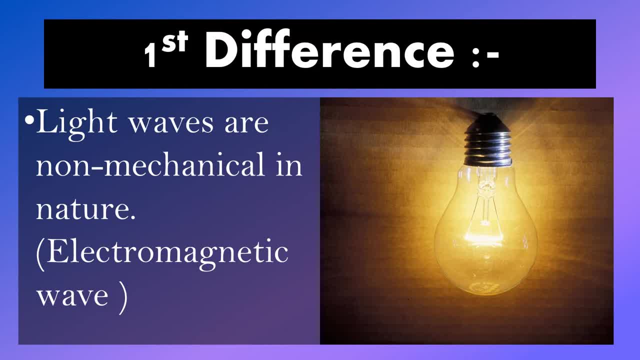 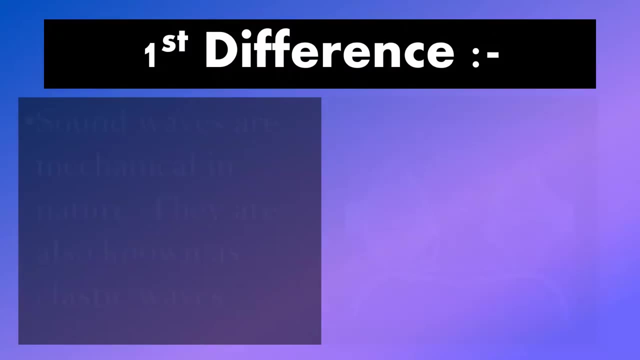 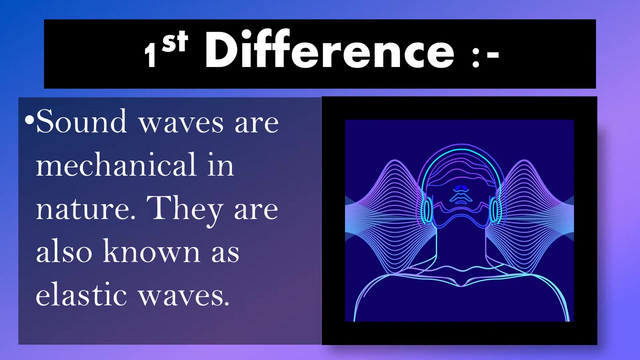 and electromagnetic in nature. This means that they don't require any material medium for their propagation. They can even travel through vacuum, which is how the sun rays reach the earth. Now, sound waves, which are elastic waves, are different, as they are mechanical in nature. They do require a material medium for their propagation. 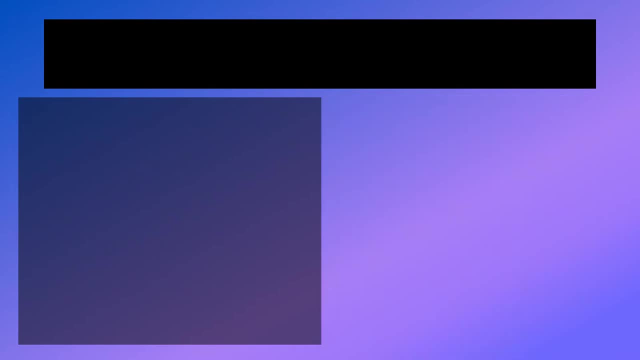 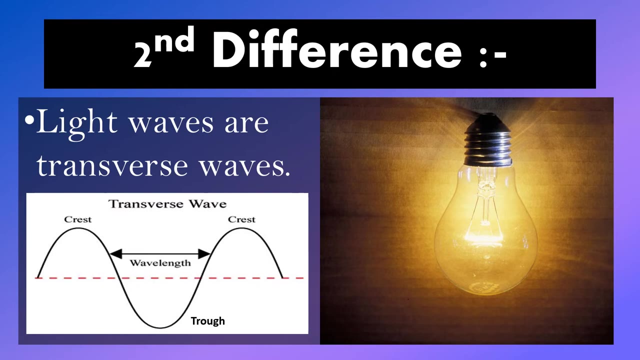 And they cannot travel in a vacuum. Now, another difference between light waves and sound waves is that light waves are transverse waves. A transverse wave is a wave whose oscillations are perpendicular to the direction of the wave's advance. Transverse waves consist of: 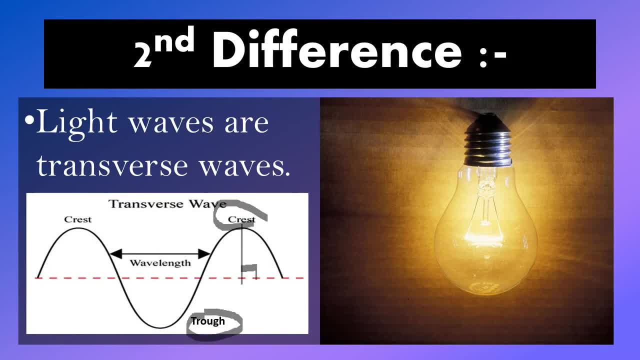 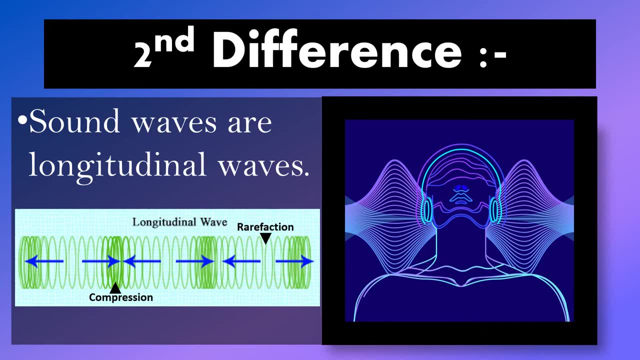 crests and rows. Now sound waves, on the other hand, are longitudinal waves. Longitudinal waves are waves in which the vibration of the medium is parallel or along with the direction the wave travels and the displacement of the medium is in the same or opposite direction of the wave propagation. 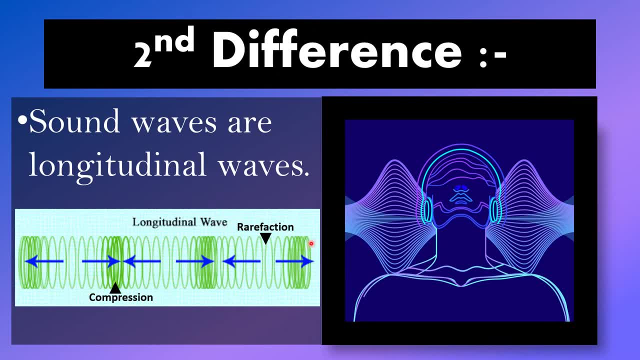 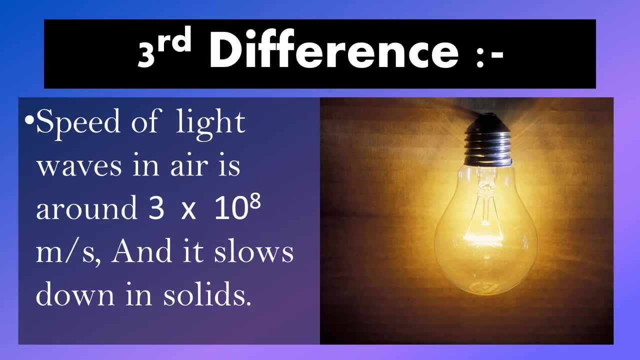 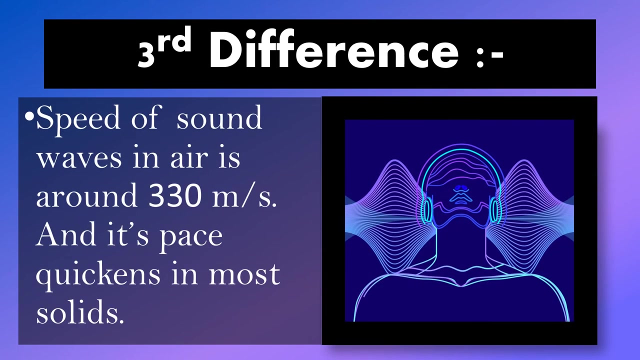 And it consists of compressions and rarefactions. Now let's look at the third difference between light and sound waves. The speed of light waves in air is around 3 x 10 to the power of 8 m per second, and it slows down in solids. Now the speed of sound waves in air is around 330 m per second. 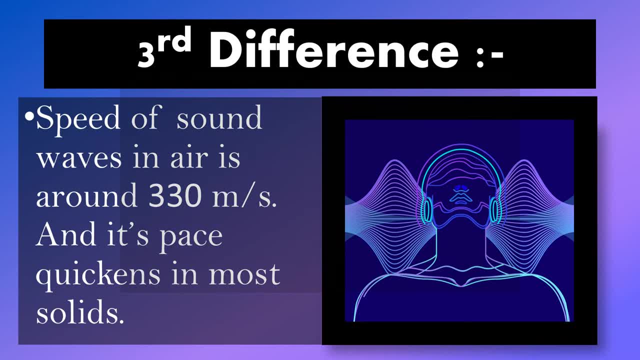 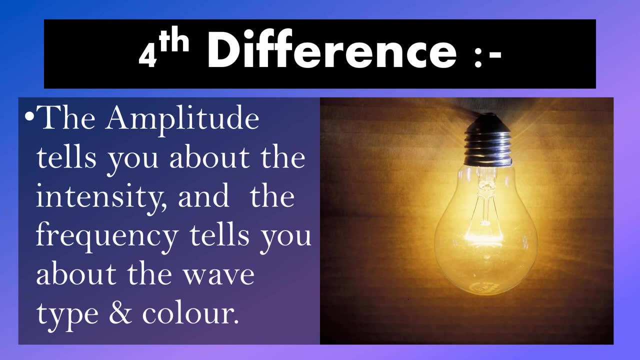 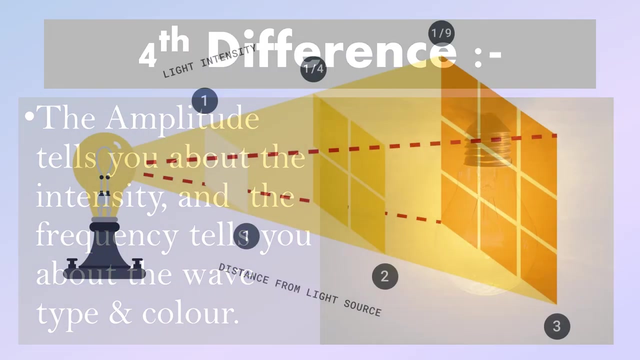 space quickens in more solids. This is the reason we always see the lightning flash before hearing the sound of the thunder. Another difference between light waves and sound waves is the use and the meaning of the terms amplitude and frequency. In light waves, the amplitude tells you about the intensity of the light and the frequency